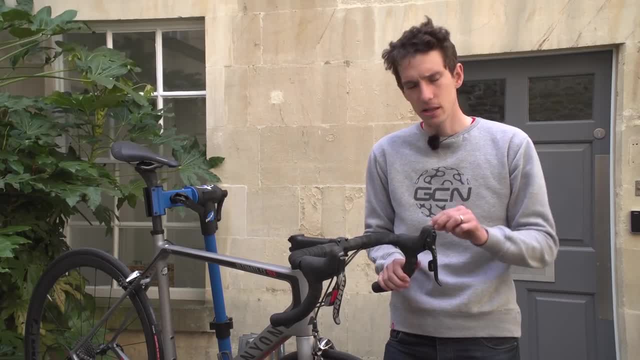 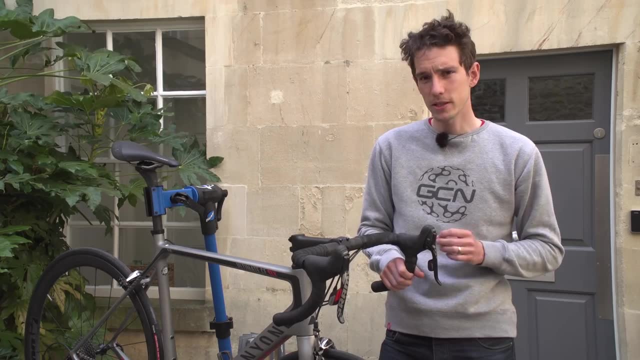 We had a question recently from a viewer about how they should go about servicing their shifters, And it's a really good question because on a road bike, these are probably some of the most complex components that you have, Although, funnily enough, I've been trying to think and I can't actually remember ever having broken a set of shifters. 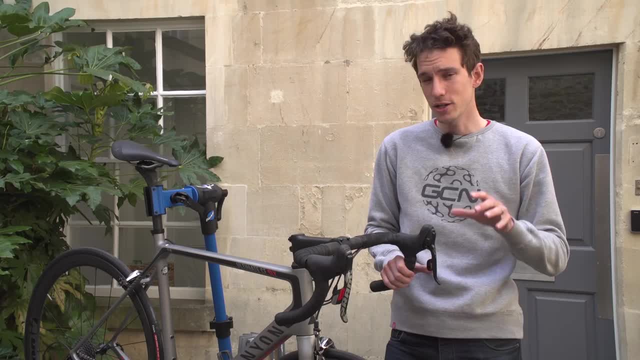 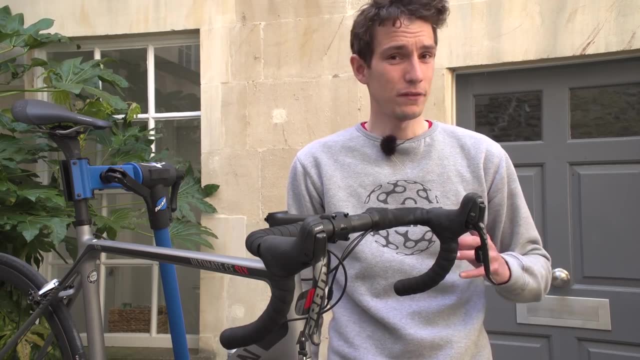 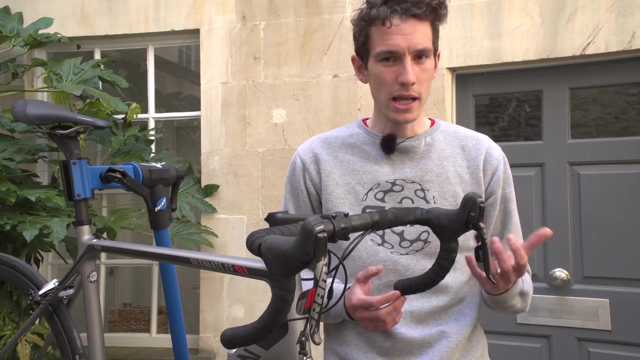 They are really robust, but that doesn't mean that you should neglect them. So here is how to service your shifters. Now, the first point is that you don't actually have to do all that much, And then, when you do something, keep it really simple, because all we're after is just to flush out any dirt or grit that might have made its way into the shifter, and then any old, contaminated and crusty grease that might have gone solid in there. 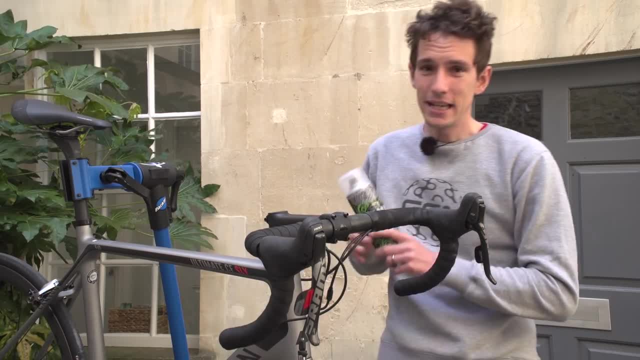 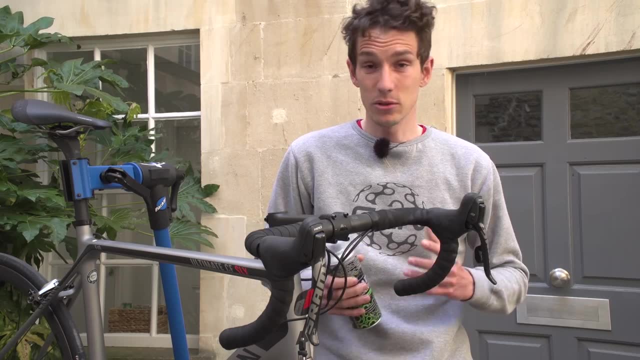 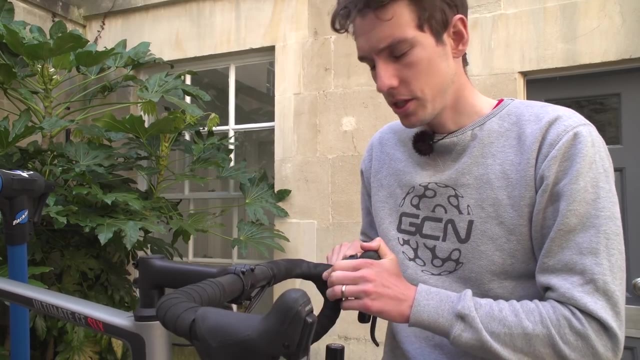 And so to do that, what we need is, ideally, an aerosol evaporative degreaser like this one, or, if you don't have that knocking around, then a solvent-based lubricant is also going to do the job. We need to remove the lever hood now to get the best access that we can to all the shifters. 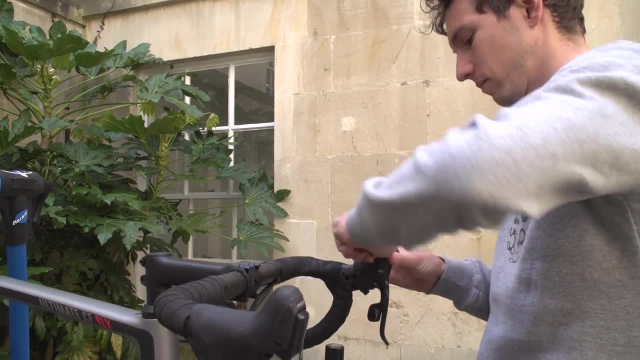 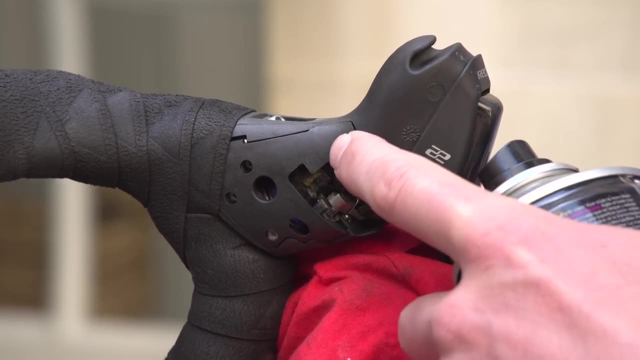 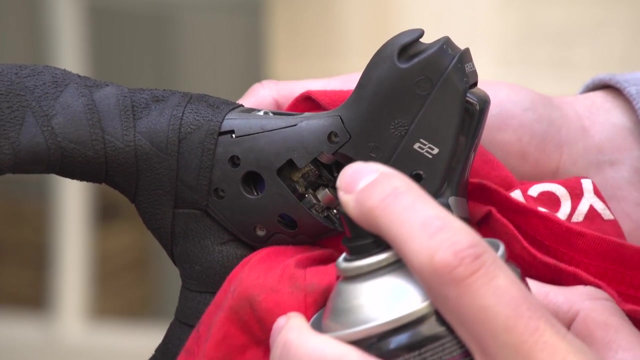 We need to remove the shifter internals. With this SRAM lever you can actually remove even more of the lever body with just four Phillips screws there. But for this we can do without. Then it's just a case of spraying our degreaser. 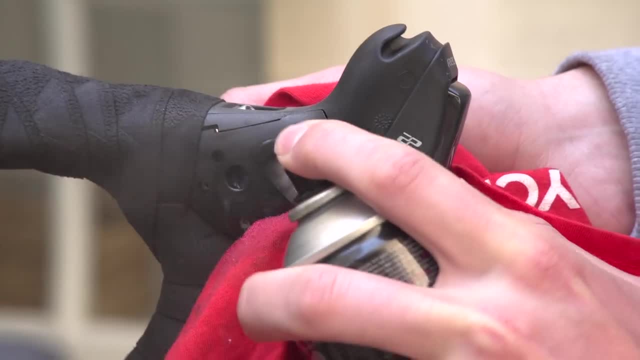 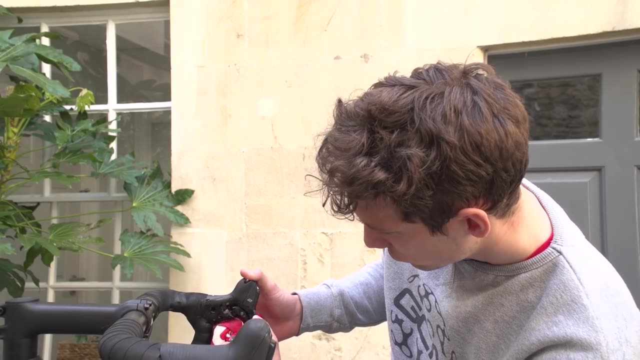 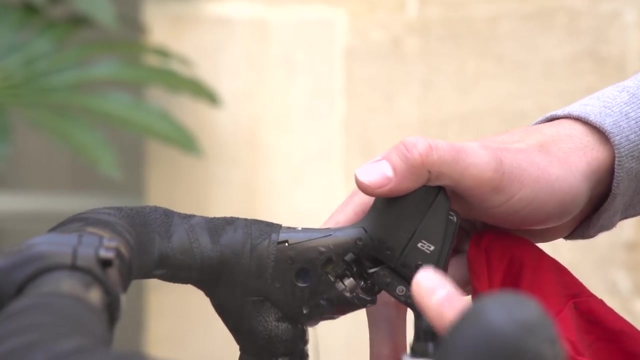 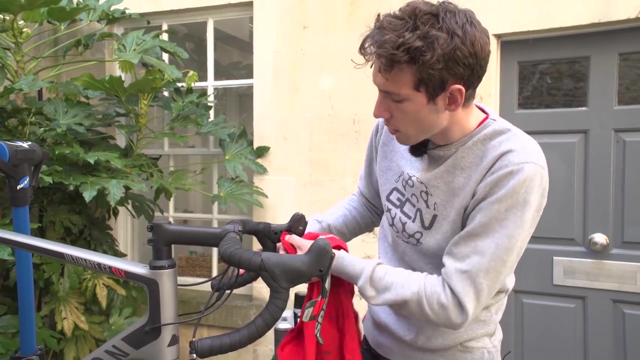 in and flushing out all of the dirt and grit and old grease as well. Don't be shy. There we go. Once you've finished and you're sure that that is clean as a whistle, then just dry it off, mop up any excess and then simply put some lube on it. 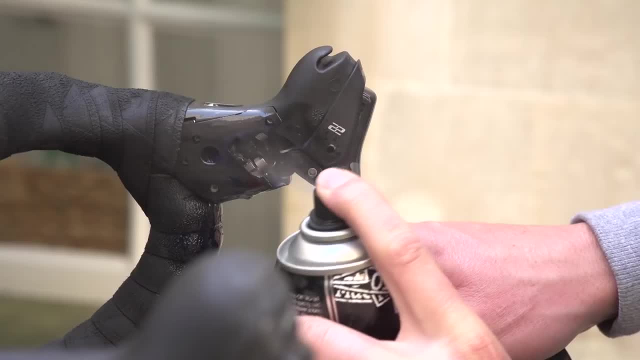 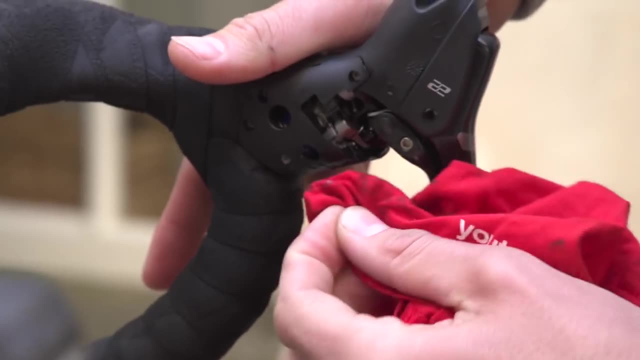 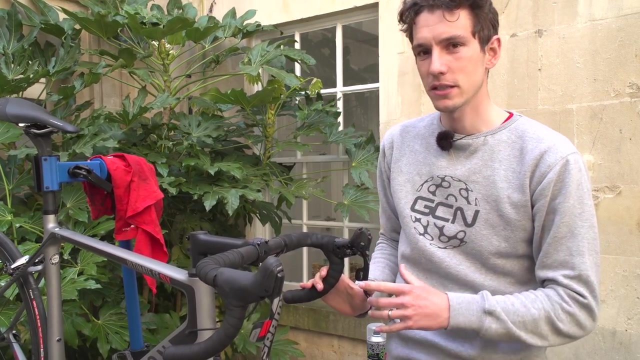 So some really lightweight aerosol lube with a bit of PTFE in it. Now, before we put the lever hood back on, it's a good idea just to put a little dab of grease on any moving parts that you can see. 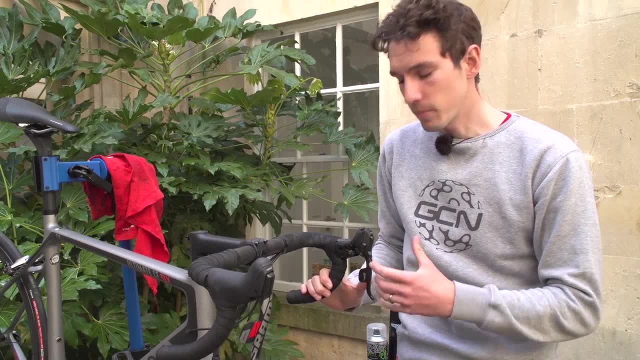 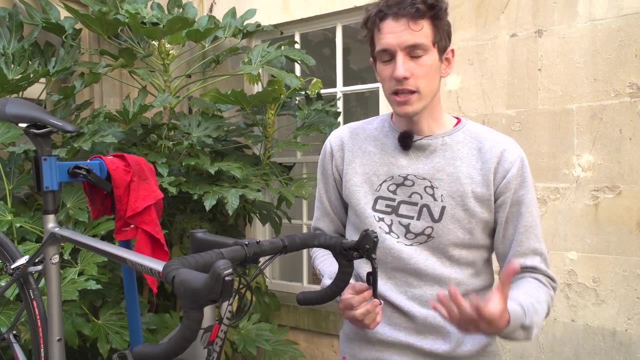 particularly on something like this SRAM lever, where you've got access to more moving parts. It just gives a little bit more weatherproofing. Now, how often should you do this procedure? Well, of course, it depends on where you ride and how much you ride.